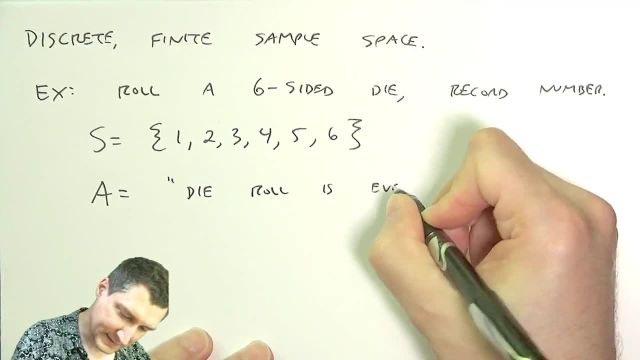 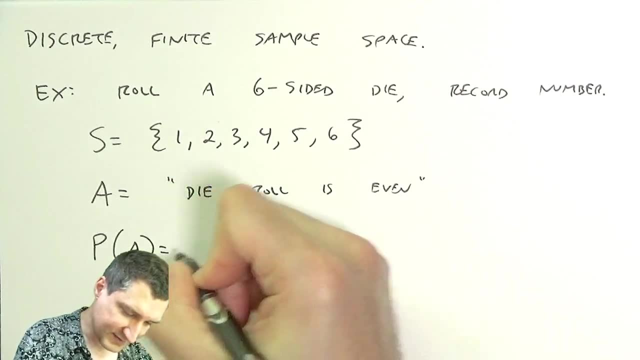 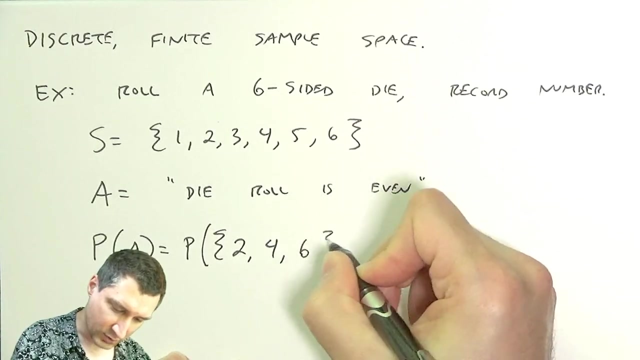 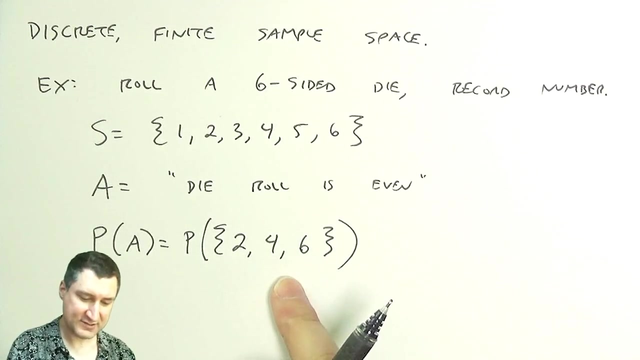 the die roll is even Okay. what's the probability of this event? Well, the probability of this event is the probability of getting two, four or six. Okay, now we know that, from what we talked about last time, this event we could take it apart into each of its individual outcomes, each of 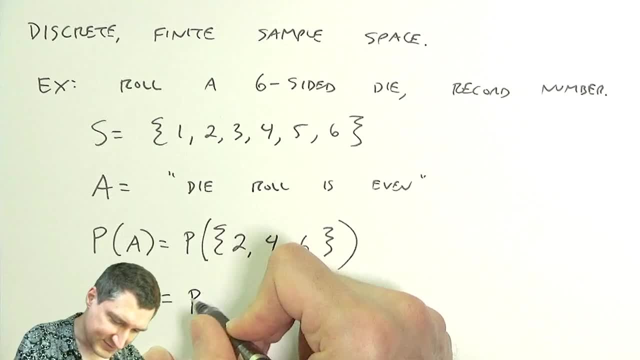 which is a disjoint event, right? So we could say that this is equal to the probability of rolling a two plus the probability of rolling a four plus the probability of rolling a six. Okay, now, this is easy to do when we have discrete. 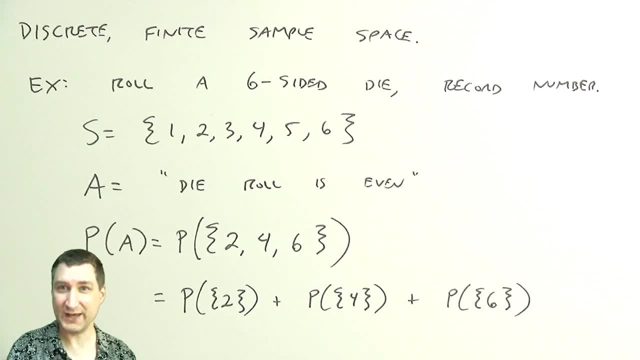 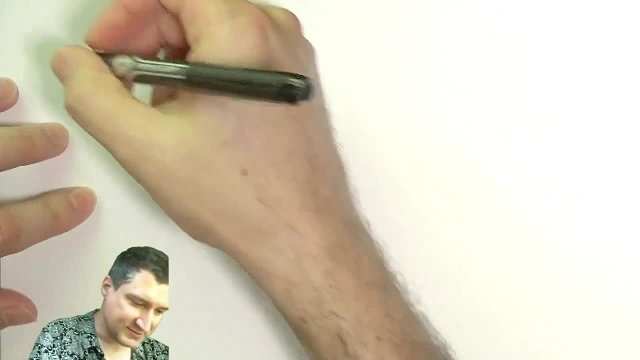 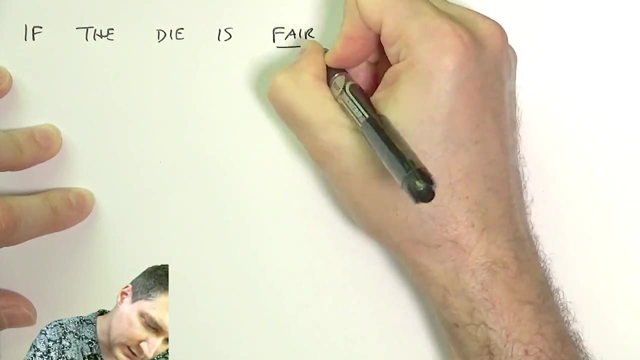 sample spaces. When you have continuous sample spaces, it's not so easy to do that. We'll talk about that in a future video, But for the moment let's think about what the probability actually should be right. So one thing you see all the time is: if the die is what's called fair, then each 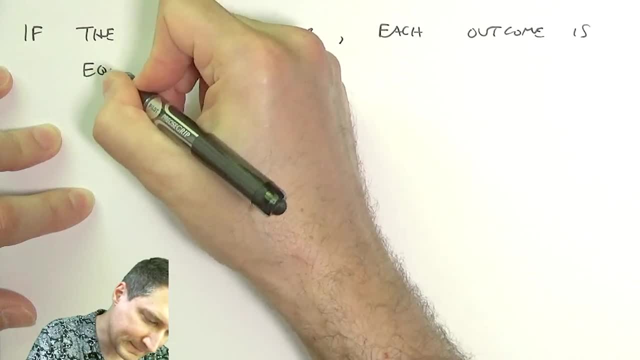 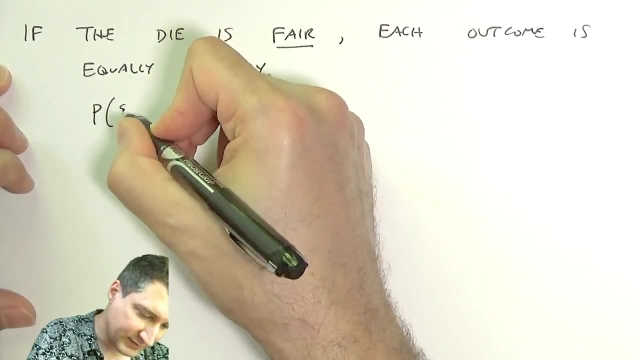 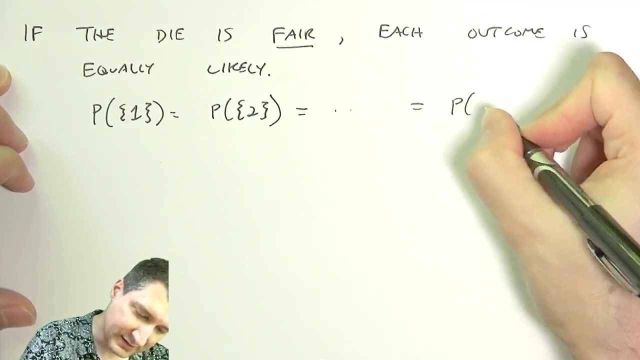 outcome is equally likely. What that means is that the probability of getting one has to be equal to the probability of getting two. This all has to be equal to the probability of getting six. these six outcomes all have to carve up the sample space fully. 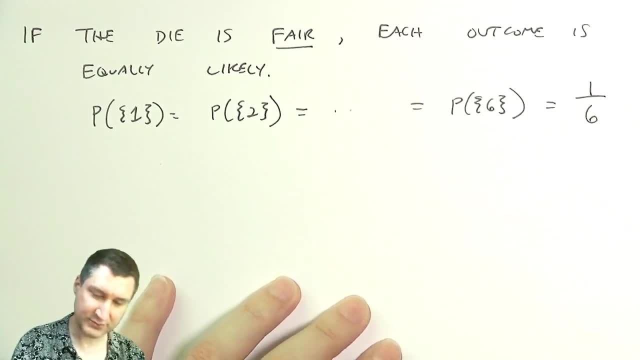 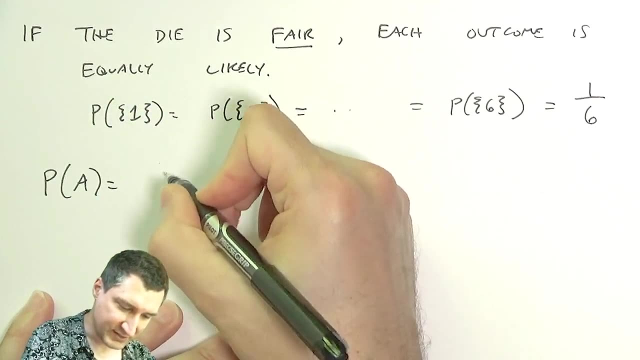 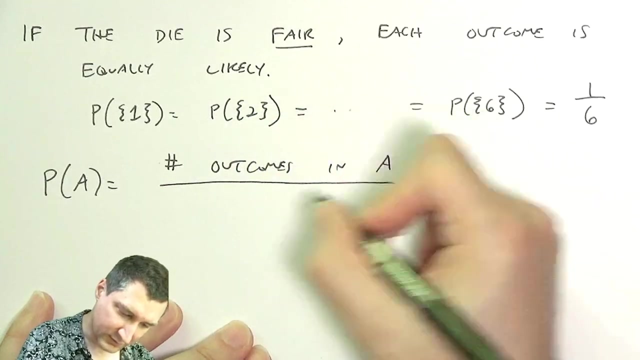 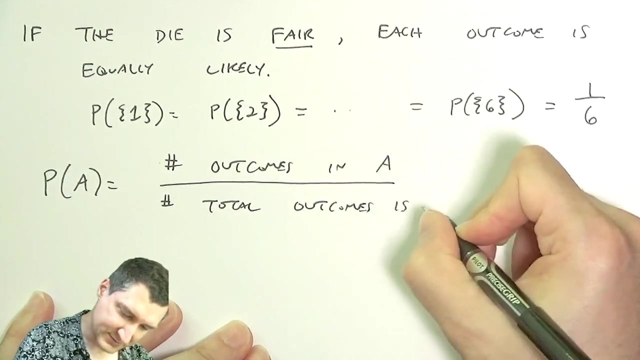 and that means that the probability of each of these things has to be equal to 1 sixth right. And we can go back and say: well then, the probability of A is really nothing more than the number of outcomes in A over the number of total outcomes in S. 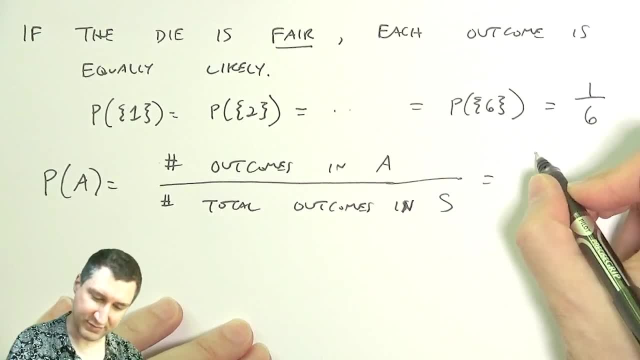 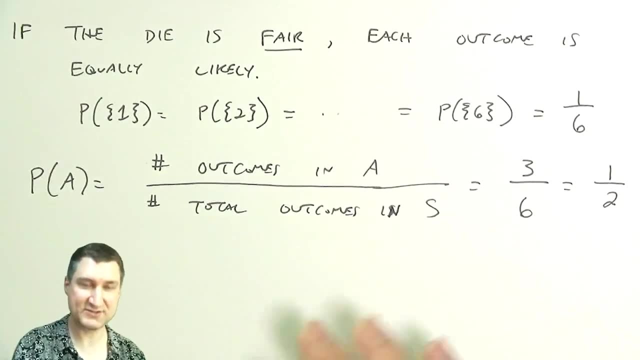 right. So in our case we have three even numbers, six total numbers, so the probability of rolling an even number is a half. Again, this only makes you know this is only true when the die is fair. right, We're going to talk about situations where not all the outcomes are equally likely. 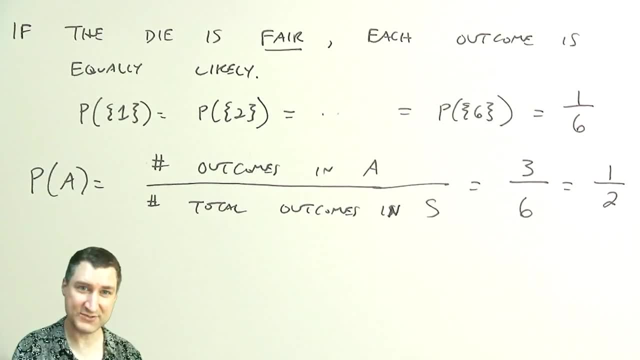 and that's a common mistake in probability- is to assume that every outcome is equally likely. We're going to talk about some examples like that in some greater detail. Okay, so this idea of kind of taking apart things into individual outcomes, we can even do when the sample space 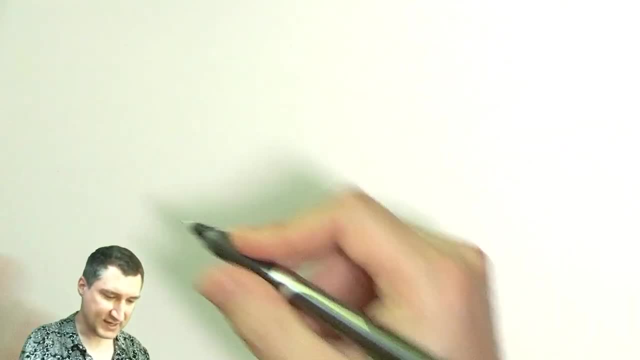 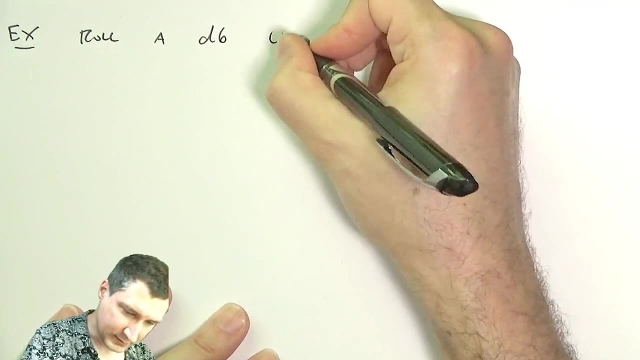 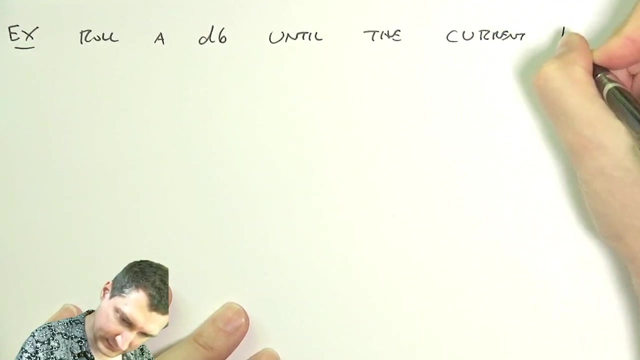 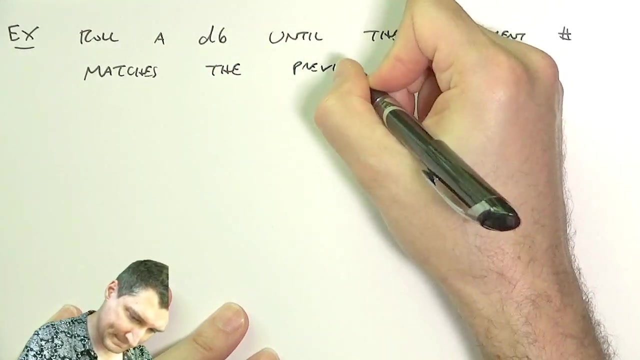 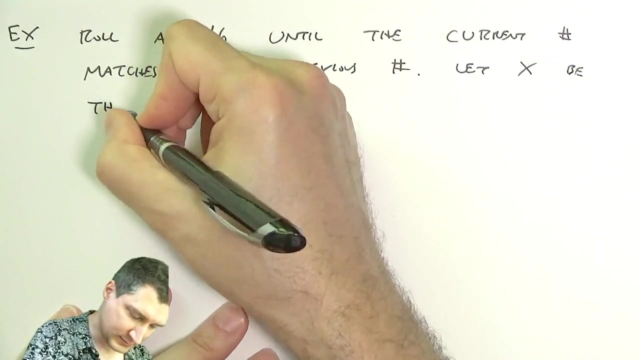 is infinite, but it takes a little bit more doing right. So, for example, we could say: roll a six-sided die. we could say y until the current number matches the previous number. Okay, And let x be that role, okay. So the sample space here is infinite. 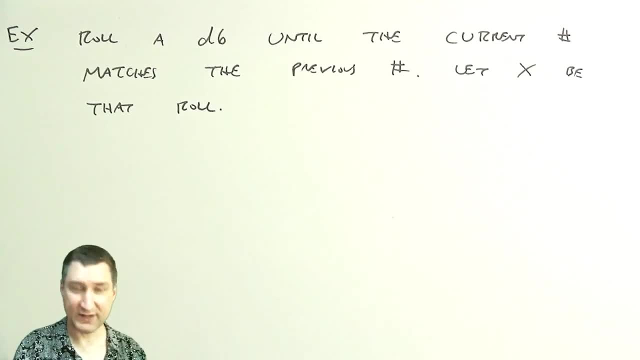 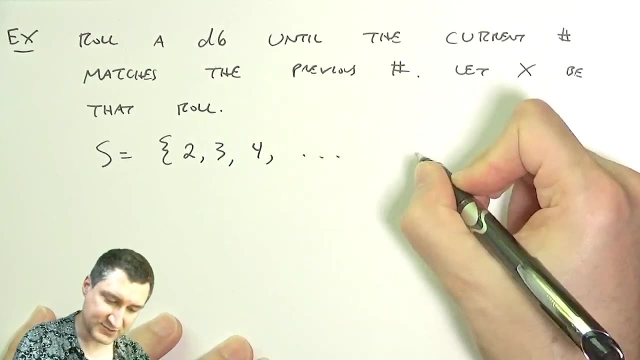 And then we can simply compute x as oraz and then we can say close here, so the earlier number is infinite right? So it could take me, you know, two rolls for that to happen, three rolls, four rolls, or I might be rolling 10,000 times and never see it happen. okay, But we can still. 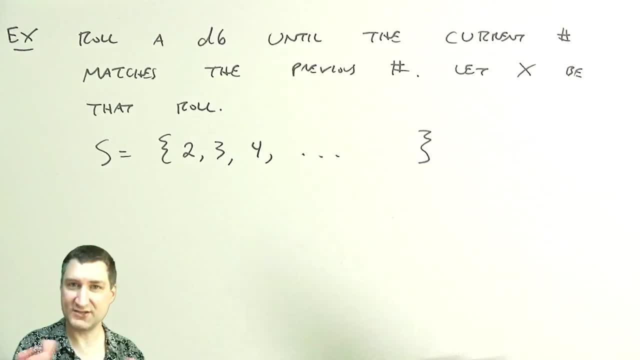 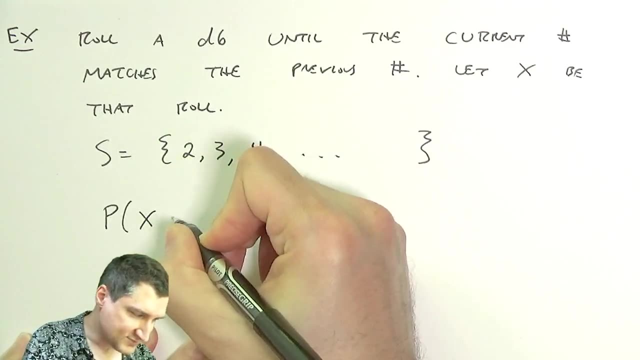 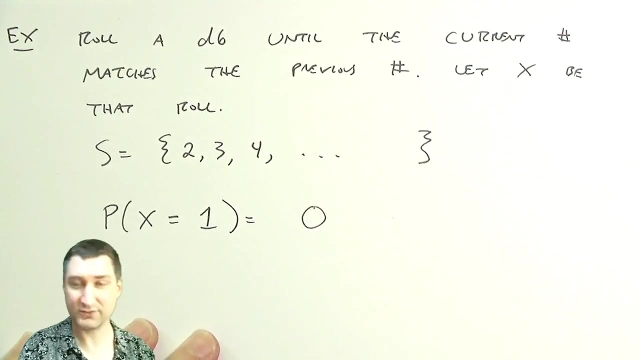 compute the probability that this value x is a certain number. okay, So let's try and actually nail down these probabilities. So the probability that x is equal to? well? here's an example. So the probability that x is equal to one is zero, right? This is not even an outcome in the sample. 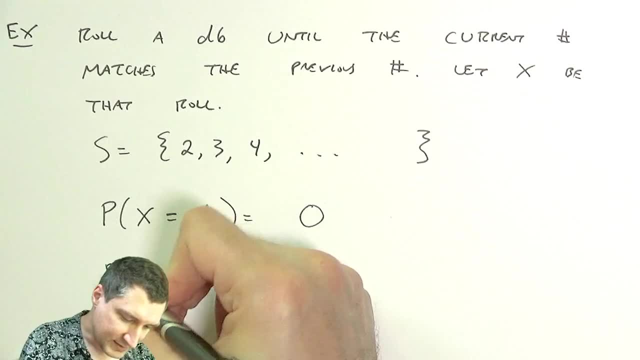 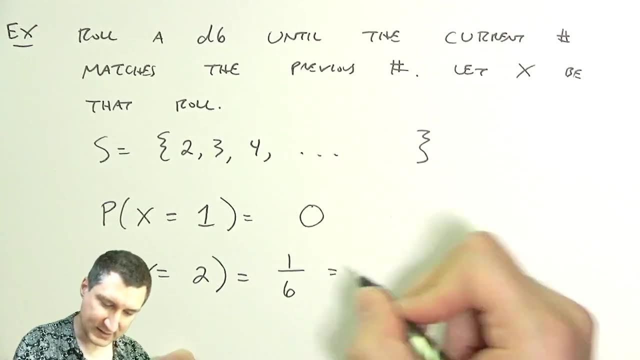 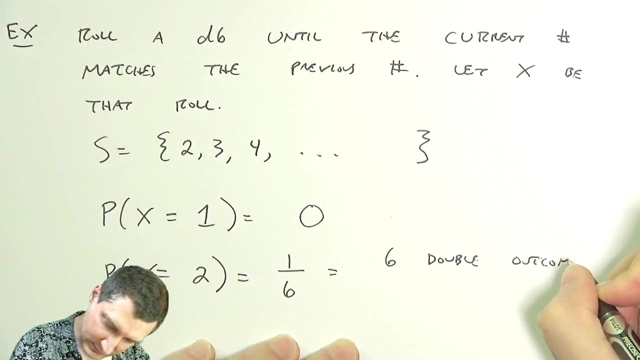 space. This is kind of like the null set, right? The probability that x is equal to two is one sixth. Why is that? Well, that's like saying that I have six double outcomes over 36 possible outcomes, right? If I look at the pairs of first die comma, second die, there are six. 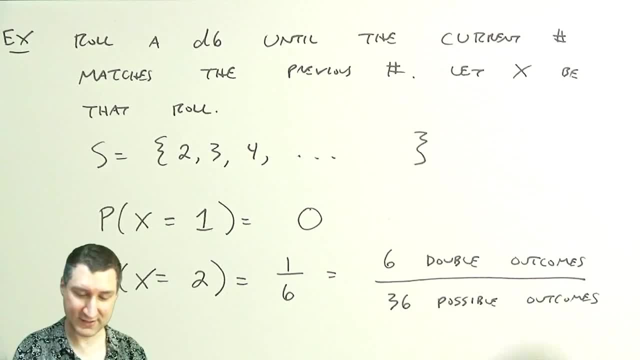 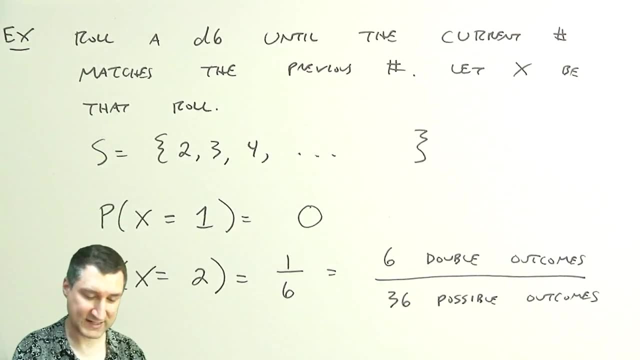 outcomes that are good and three outcomes that are bad right. So that means that the probability of getting it kind of on the second try, you know, the first time you can possibly get it is one sixth right. The next one is a little bit trickier right And I apologize, this is 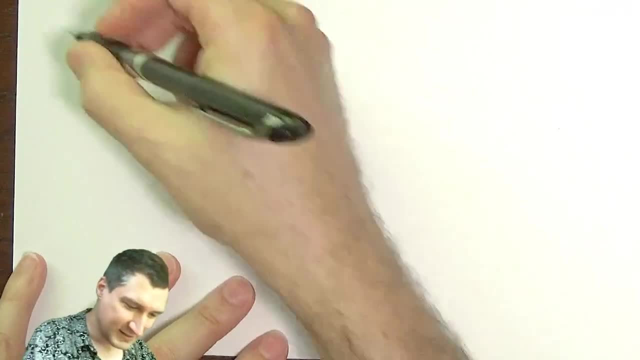 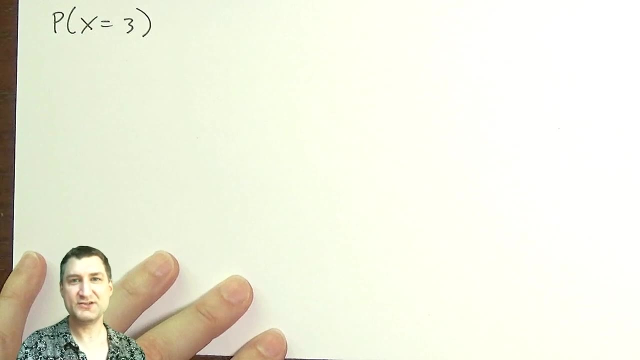 this way. probably it's behind my head there. Sorry, I have to watch my head. So what is the trickier? What we need is that roll three has to be the same as roll two, but I can't have already had roll two be the same as roll one. So in some senses it's like saying I failed on roll two and 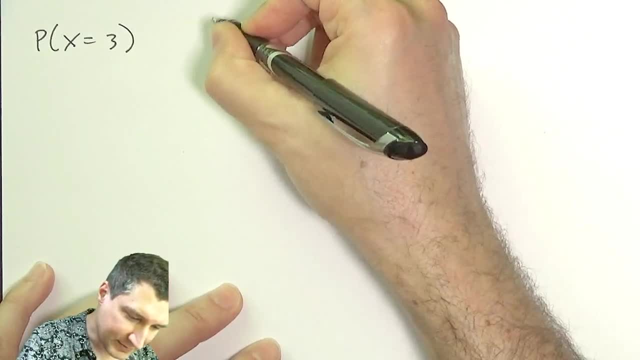 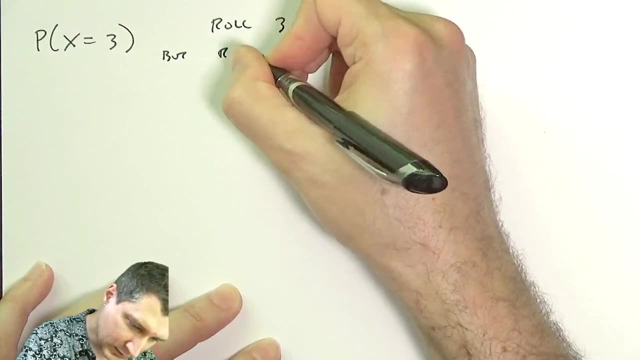 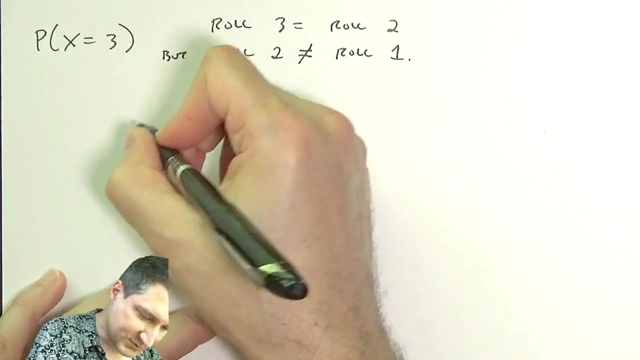 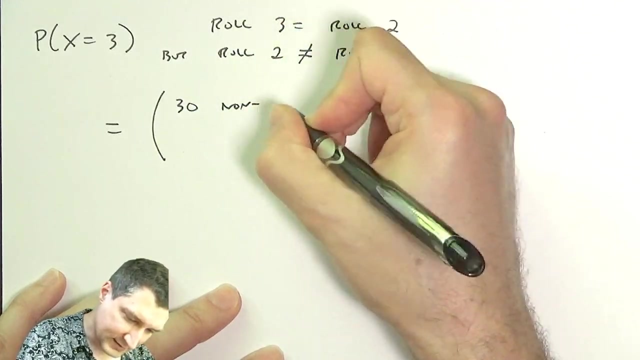 I succeeded on roll three, right, So roll three equals roll two, but roll two was not equal to roll one. okay, So what's this? So what's the probability? Well, this is like saying that on roll two I got 30 kind of bad outcomes. 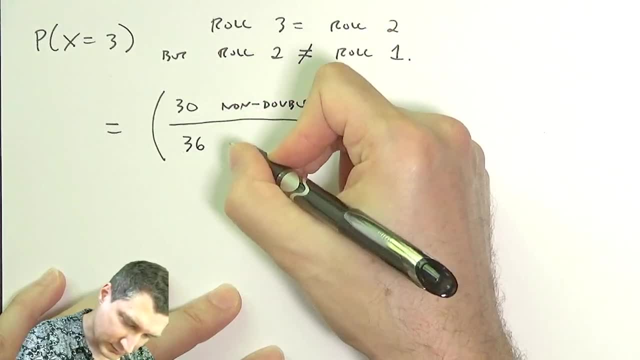 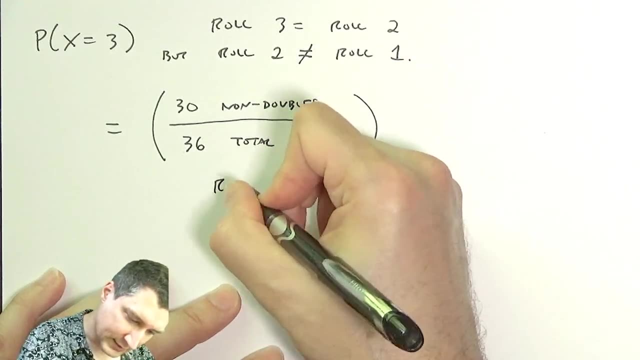 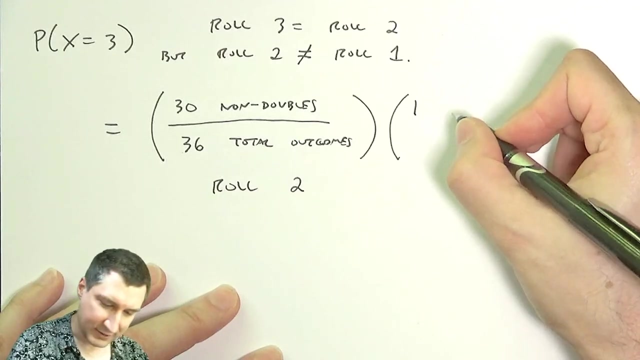 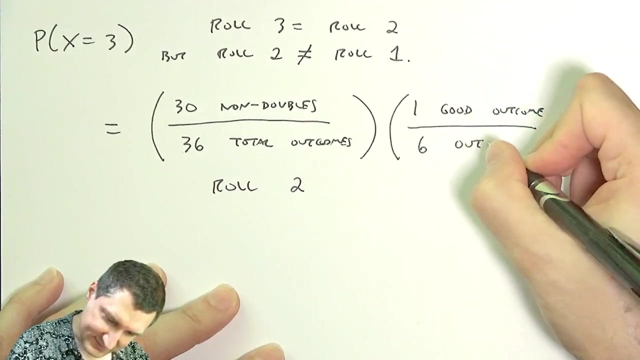 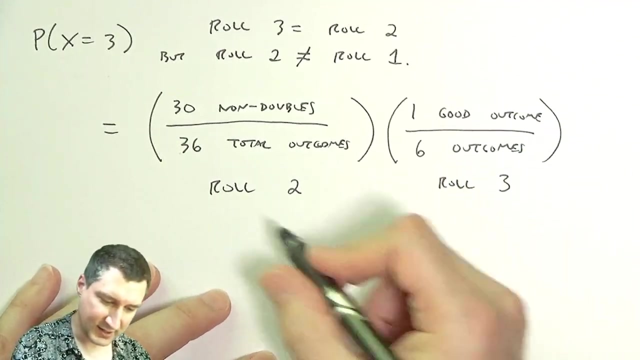 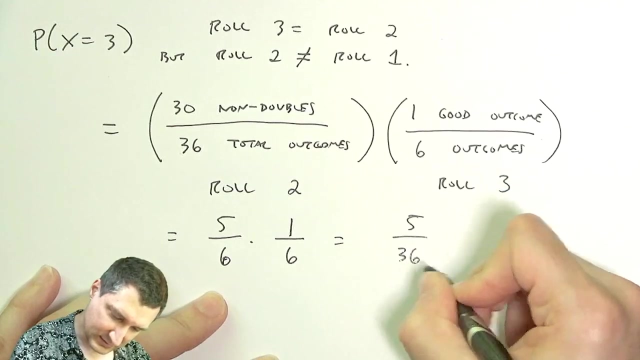 right, This is what happened on roll two And then on roll three. I have one- you know- good outcome Over six outcomes, right? This is like saying that whatever I saw on roll three matches what I saw on roll two. So here I can say that the result is five sixths times one. sixth is five thirty-sixths. 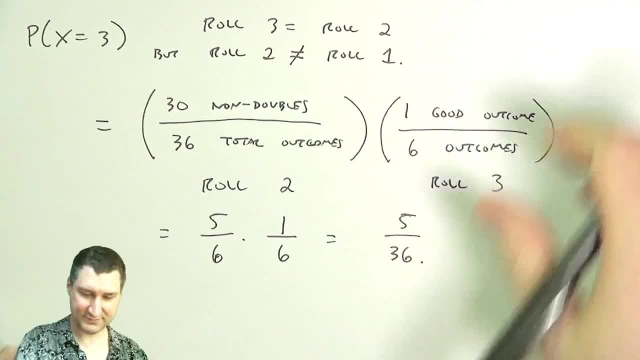 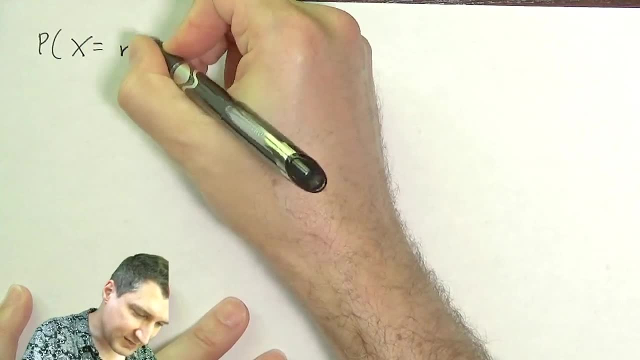 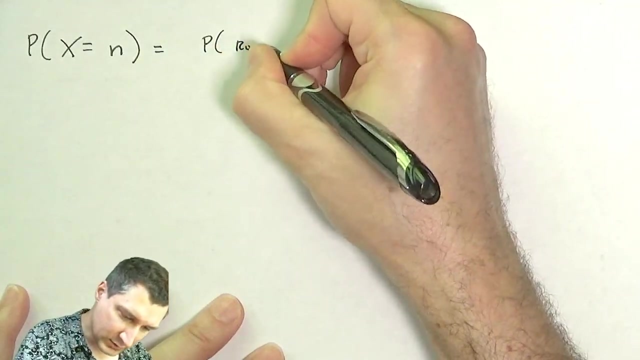 okay. So in general, what we can do is kind of pull this all together to say what is the probability that x is equal to some number n Right? Well, that's like saying the probability that roll two was not equal to roll one times the. 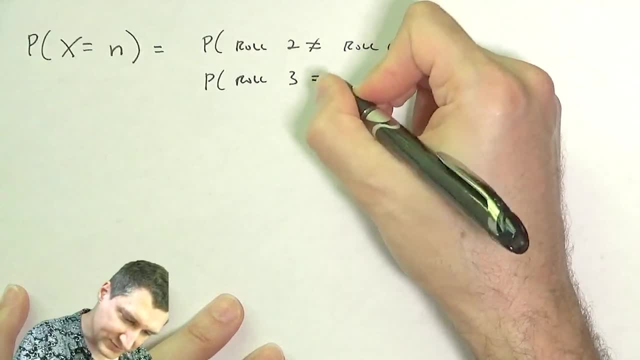 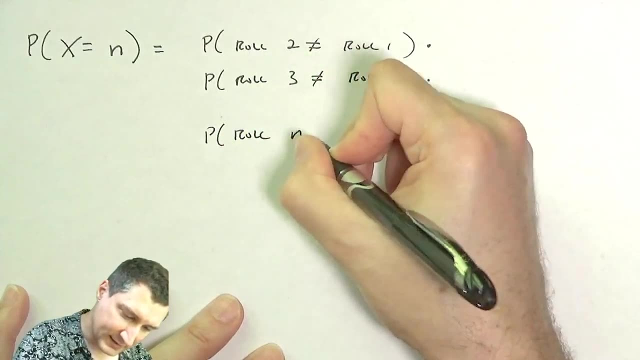 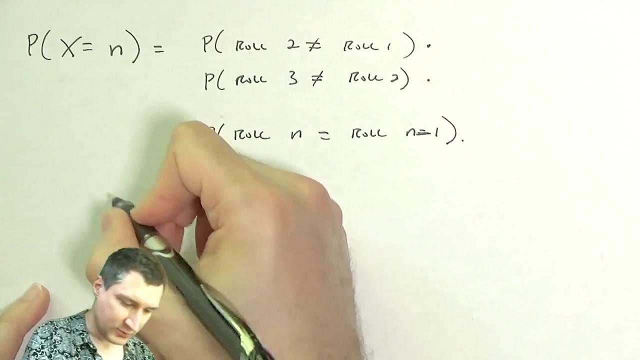 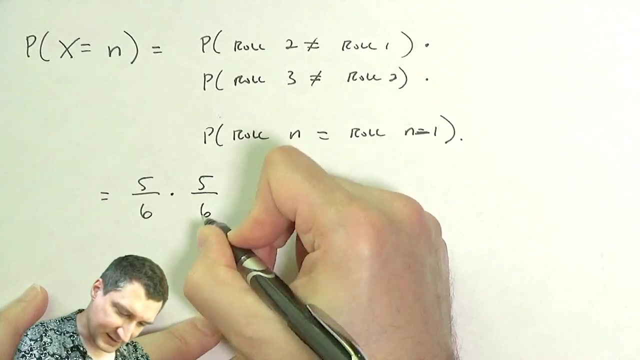 probability that roll three was not equal to roll two times the probability. dot, dot, dot. Finally, I say that on roll n I got the right answer. okay, So the probability of the first thing happening, failing on roll two- is five sixths. Then I have failing on. 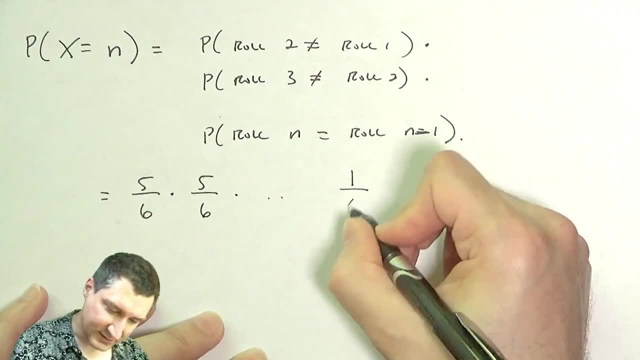 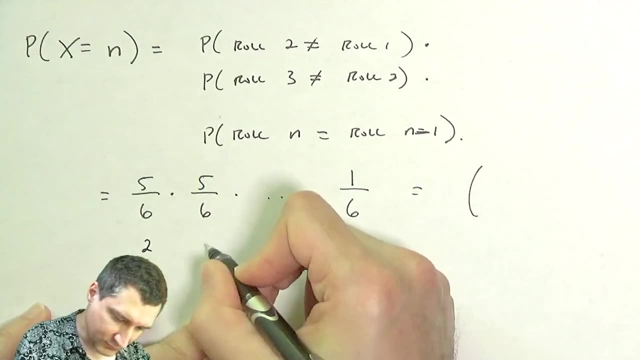 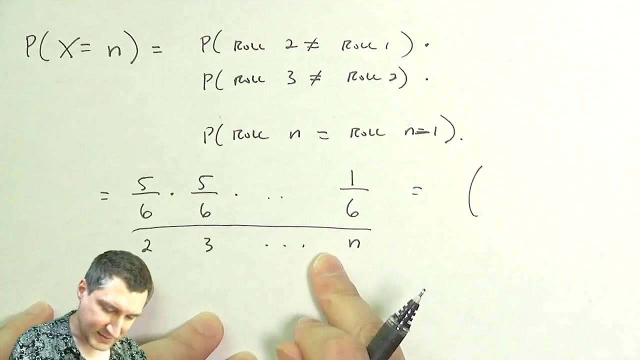 roll three is five, sixths, dot, dot, dot, all the way up to succeeding on roll n right. So here this is like saying I have roll two, roll three, dot, dot, dot all the way over to roll n, So I have n minus two failures and one failure right, So I have n minus. 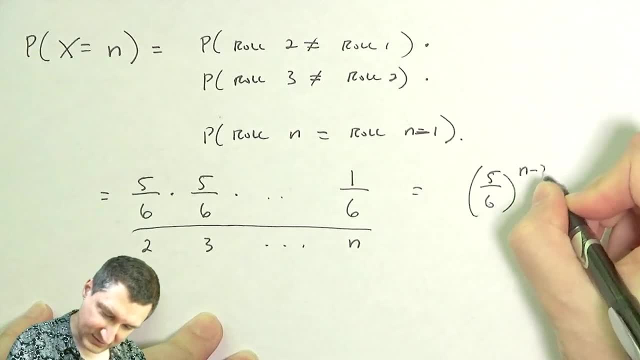 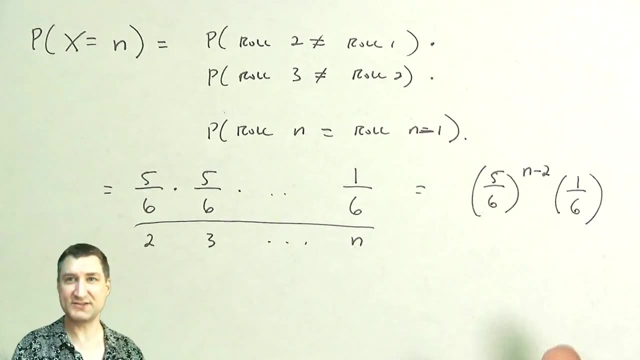 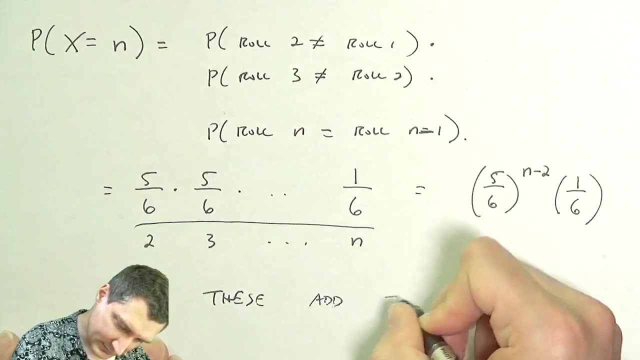 two failures and one failure, One success, okay. So here this is like saying, okay, I have characterized what happens at any possible roll, and now I should just do a quick sanity check to make sure these things add up to one, right? So do these add up to one? I sure hope so. 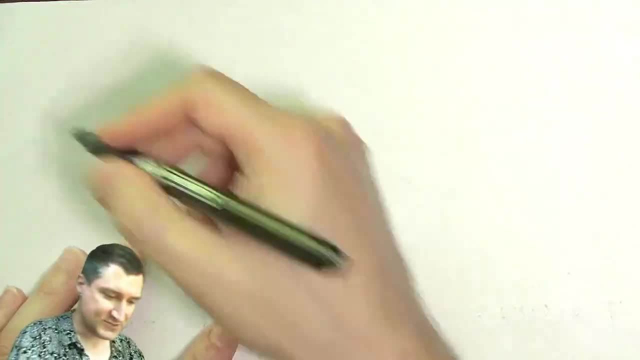 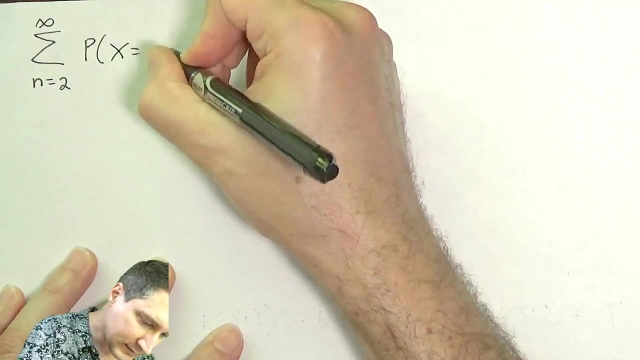 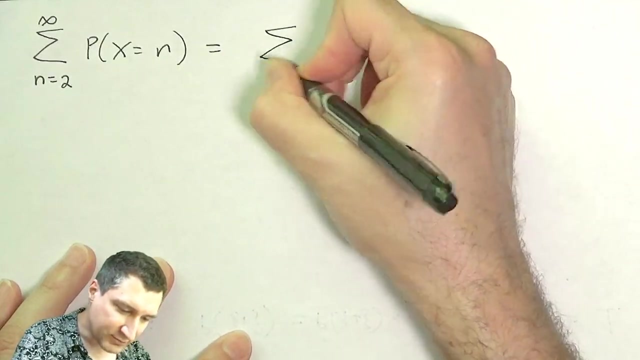 Well, again, these are all disjoint events, right? So I could be, you know, I could be looking at the probability that I got two, three, four, five, all the way up to infinity. These numbers should add up to one, and now I know a general formula for the probability. 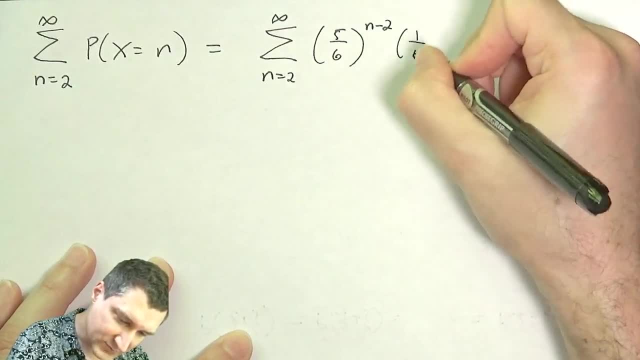 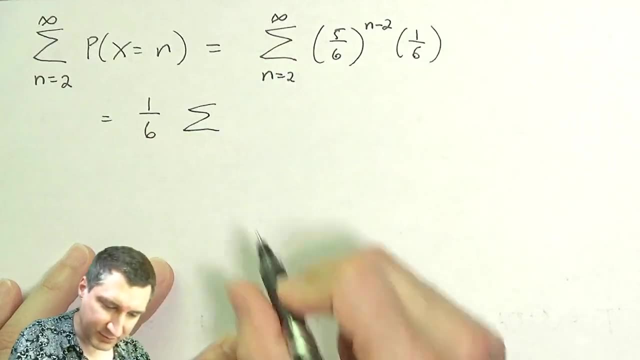 It's five sixths to the n minus two times one sixth. I can take the one sixth out and I can renumber my sum. Okay. Okay, I've made my formula. I'm just gonna do a series of 1 over 1 minus a to start at zero instead of two right. 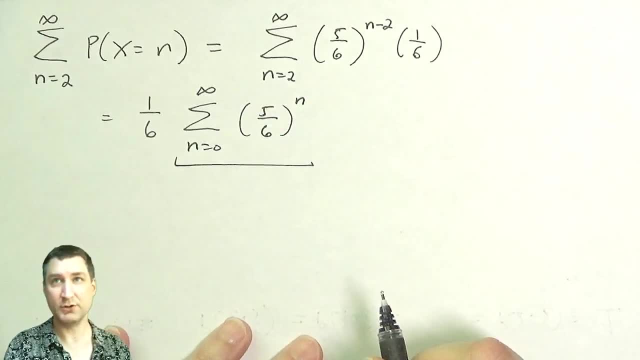 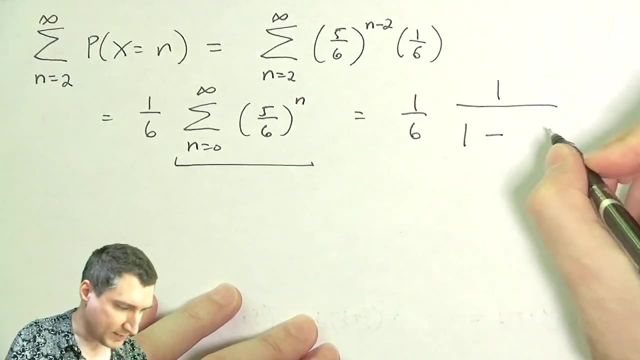 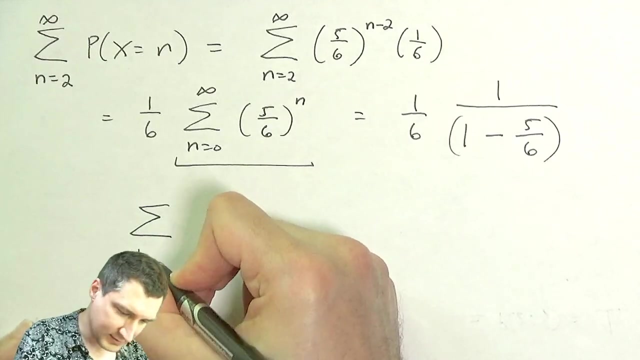 And now this is a summation formula that should be familiar to you from, hopefully, some other class, right? The answer here is 1 over 1 minus five sixth. What I'm using is this formula that says that when a is less than one, that this infinite. 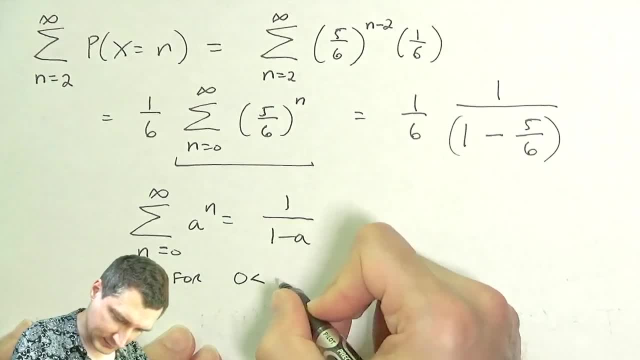 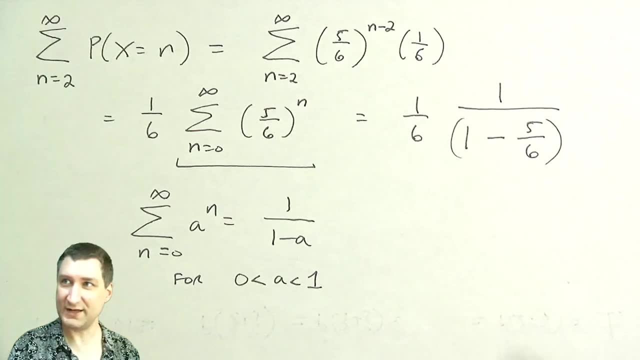 sum is equal to 1 over 1 minus a when a is between zero and one right. That's a good thing to remember. So if you took a class like signals and systems, you probably already had that written down somewhere And now I can say: 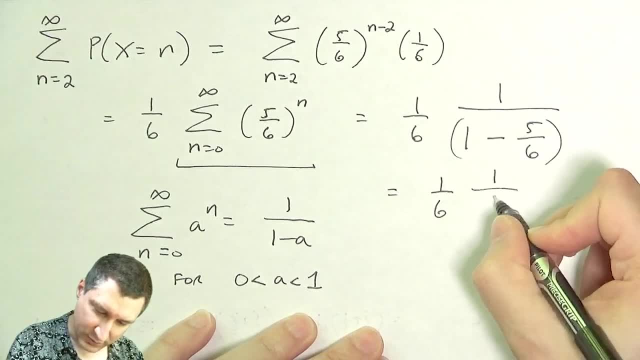 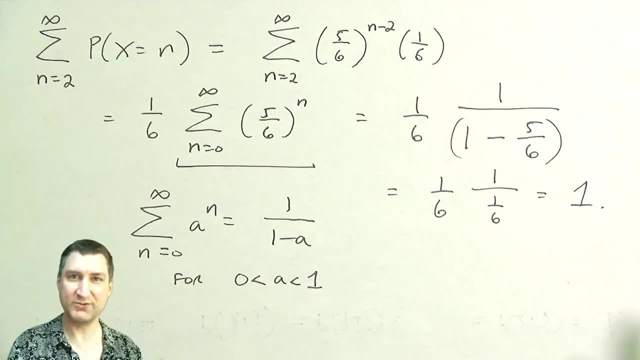 okay. well, my result in the special case is one over this, and this is just equal to one. So that's good. We showed that we got a sum of probabilities equaling to one. As we're going to talk about later on, this is a kind of an example of what's called a geometric probability. 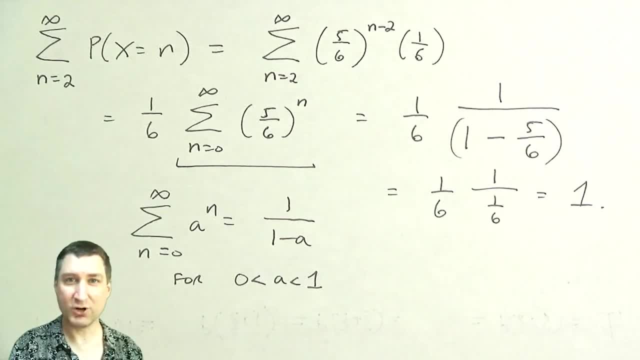 distribution. Okay, so next time we'll talk about even more complicated ways of talking about discrete probability spaces, And these are going to be the kind of combinatorics problems that you oftentimes see in probability homeworks- things like card tricks and probability of getting a. 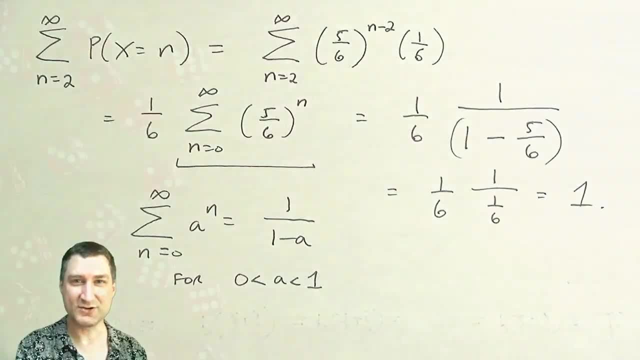 royal flush on a poker draw, stuff like that. Okay, so tune in next time for more examples. 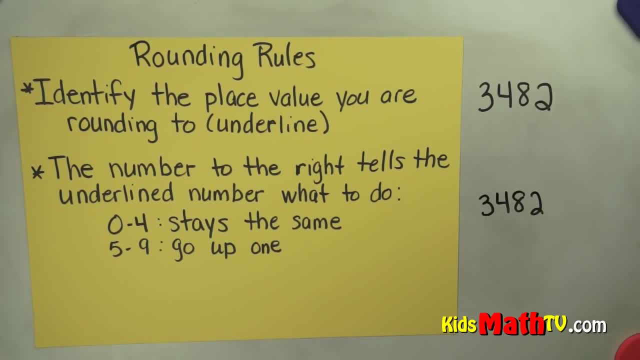 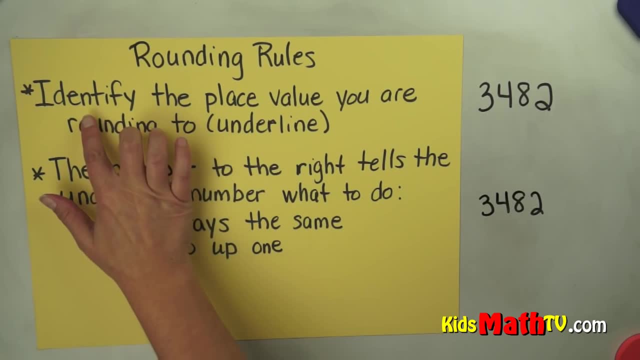 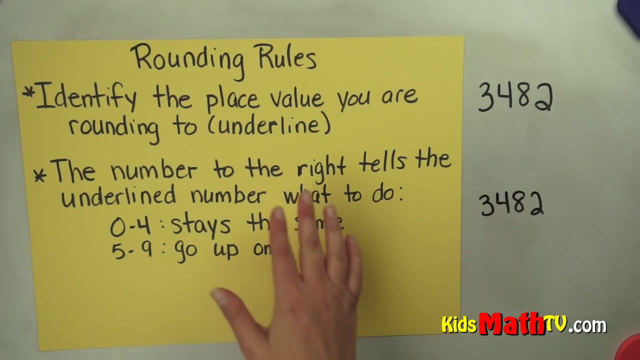 In this lesson, you will learn the rounding rules, Okay, so when you are rounding, there are a couple things to do. First, you need to identify the place value you are rounding to, and I like to underline it. Okay. then, once you determine the place value you're rounding to, the number, to the 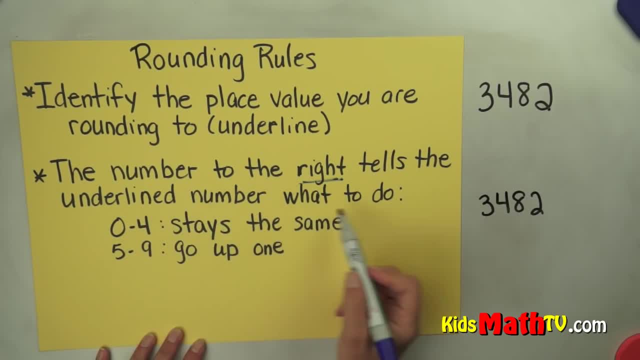 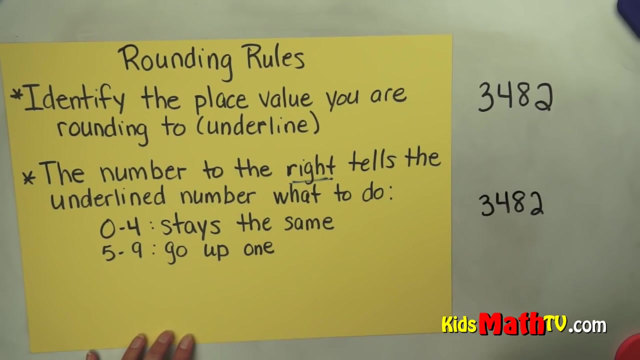 right tells that number that's underlined what to do. Okay, if the number to the right is zero to four, the number that you underline stays the same. If the number to the right is five to nine, the number that you underlined will go up one, Okay. so let's look at the example using the. 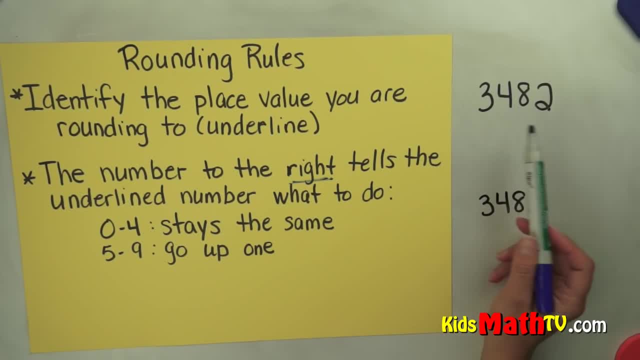 rules. Let's round this to the. let's round this number first to the nearest hundred, Okay, so first identify the place value you're rounding to and underline it. So the hundredth place is the four. Let me grab a pen that shows. So the four. that's what I'm rounding to, Okay. 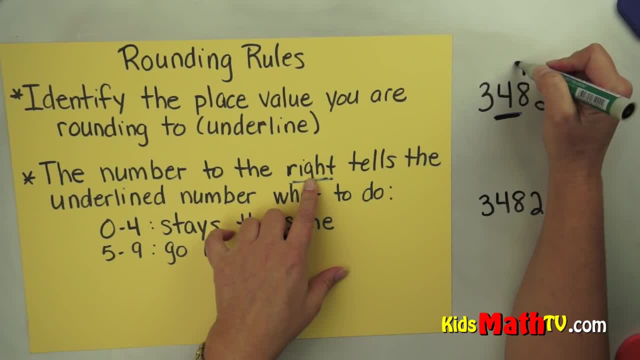 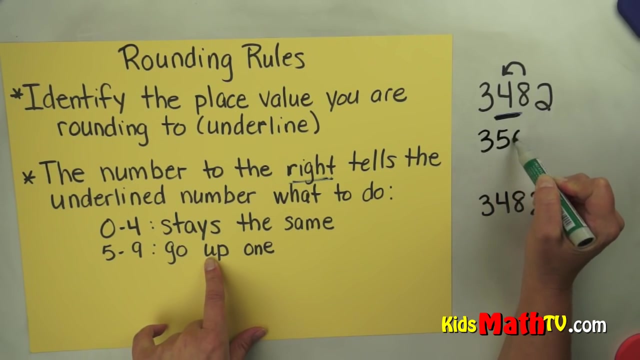 then the number to the right. this eight tells that four what to do. Well, that eight is between five and nine, so it tells that four to go up one. So this number then becomes 3,500.. Okay, which means 3,482 is closer to 3,500 than it is 3,400.. Let's try that again. We'll use the same. 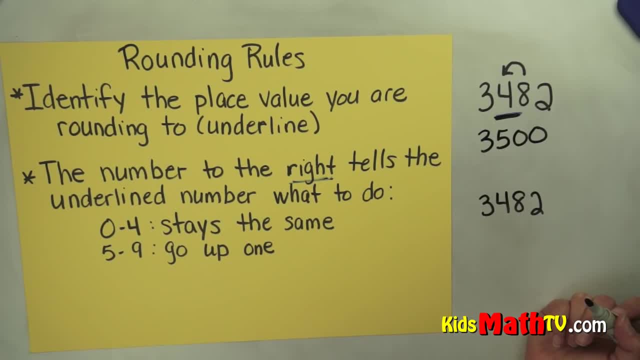 number, but this time we'll round to the nearest tens. Okay, tens. So identify the place value you're rounding to. The eight is in the tens place. The number to the right, which is the two, tells that eight. what to do? Okay, so the two is between zero and four, which tells that eight. 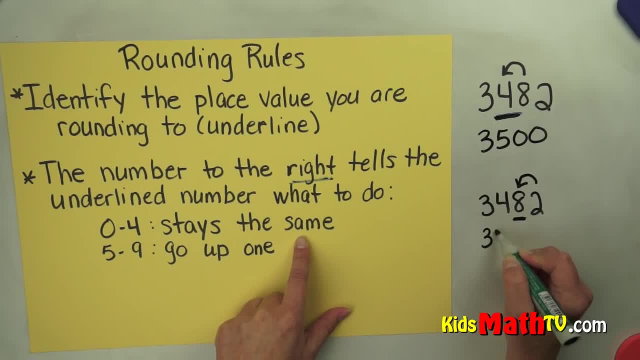 to stay the same, So this number becomes 3,480.. Okay, because this number is, let's see, 3,482 is closer to 3,480 than it is 3,490.. And that's the end of this lesson.